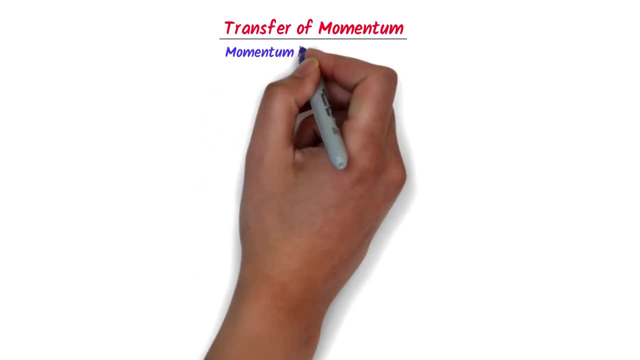 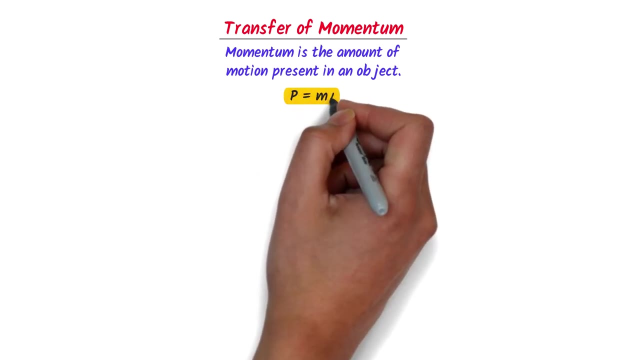 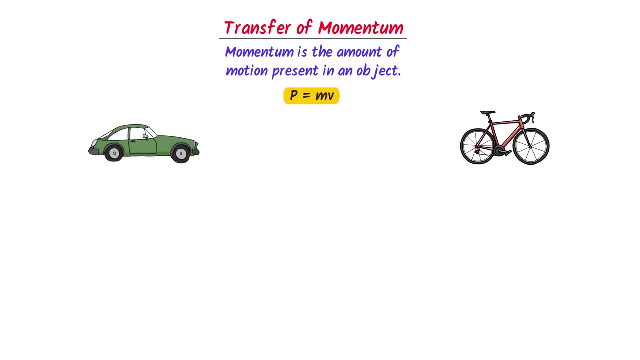 of momentum during collision. We know that momentum is the amount of motion present in an object. Its formula is: P is equal to m into v. For example, consider a moving bicycle and a moving car. Let they both move with a velocity of 40 meter per second. We say that the momentum of the bicycle is smaller and that 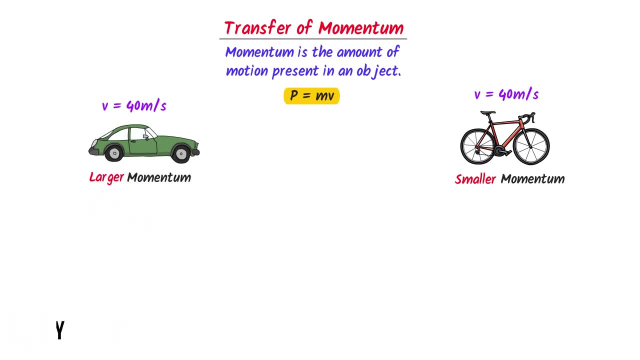 of the car is larger due to the difference in size. Or we say that the bicycle has less amount of motion and the car has more amount of motion. Simply remember that when there is motion, there is momentum. No motion means no momentum. Let me repeat it: When there 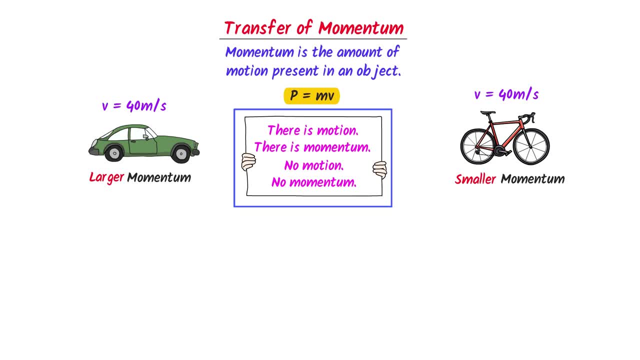 is motion, there is momentum. No motion means no momentum. In this lecture, for simplicity, in case of momentum, I will use the term motion, which students easily understand. Now consider two balls. Let this ball is stationary. our momentum is zero While this ball is moving. so it possesses momentum due to its motion. Now this 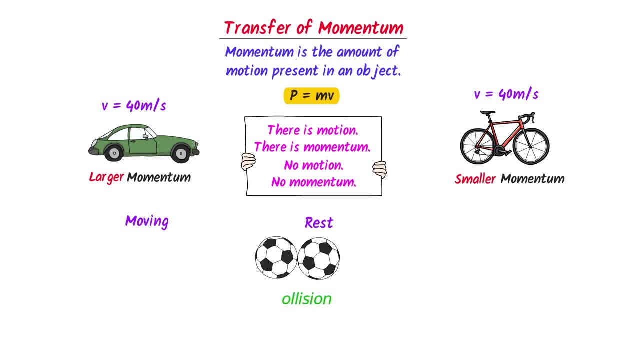 moving ball will collide with the stationary ball. After collision, the moving ball will stop and the stationary ball starts moving. Here listen carefully. During collision, the moving ball has transferred its momentum to the stationary ball. That's why it starts moving. Let me 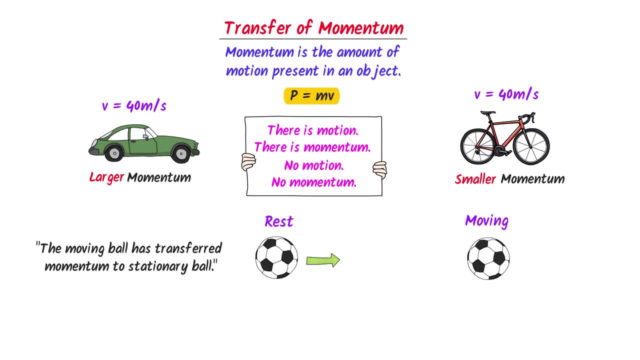 repeat it: During collision, the moving ball has transferred its momentum to the stationary ball. That's why it starts moving. Therefore, remember that when particles collide, they transfer some sort of momentum. So note it down, this concept, which we will use in Heisenberg uncertainty. 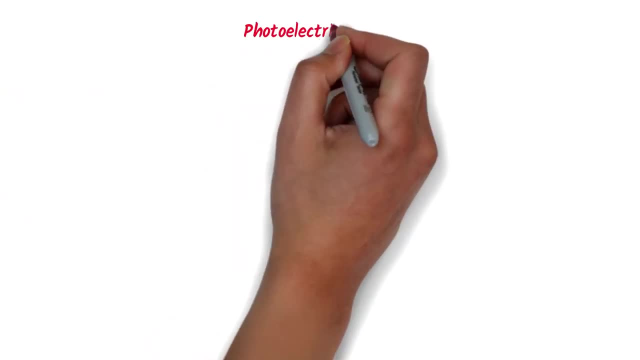 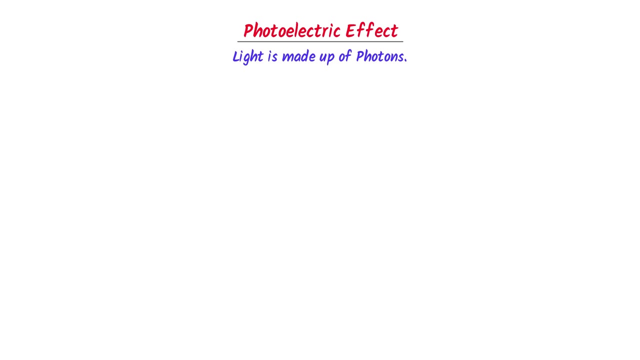 principle. Secondly, we should also learn photoelectric effect. We know that light is made up of photons, just like we human beings are made up of cells. Now, according to dual nature of light, light or photons can act as a wave, and light or photon can act like a particle, For example. 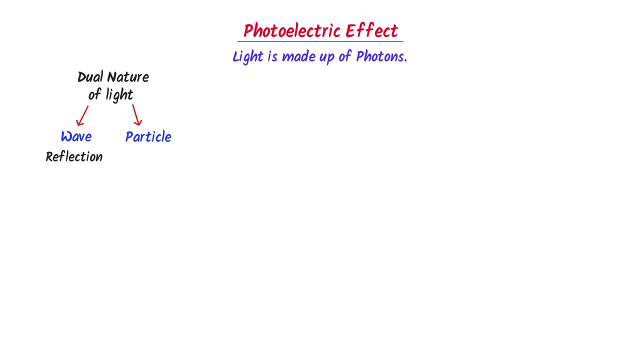 light or photon is reflected when it hits any surface, So it is a wave nature. Secondly, photon transfers momentum during collision, like the one we learned in the previous example, So it is a particle nature. To learn it more simply, let's consider a metal. 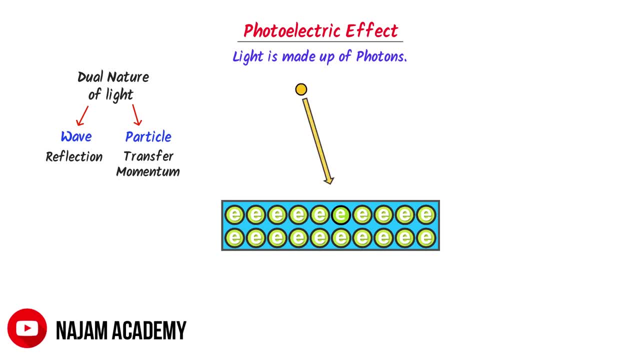 surface. Now light is incident on this metal surface. The single photon of light will hit this electron During collision. the photon will transfer its momentum to this electron. As a result of this, the electron is ejected from the metal surface. That's why we call 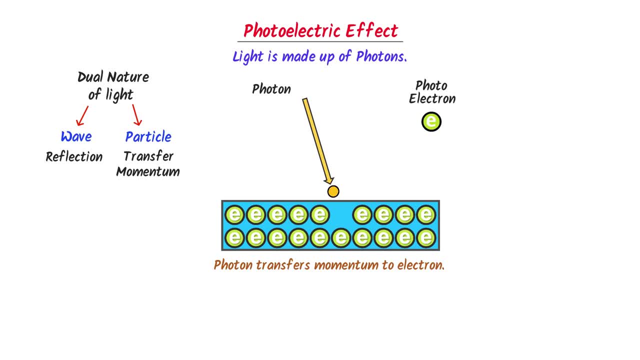 it photoelectron. Now listen carefully: During collision, photon changes the position and momentum of an electron. Let me repeat it: During collision, photon changes the position and momentum of an electron. Remember that photon only changes momentum of microscopic particles like electron. 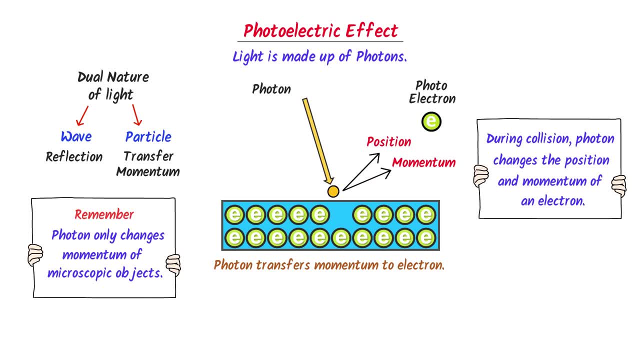 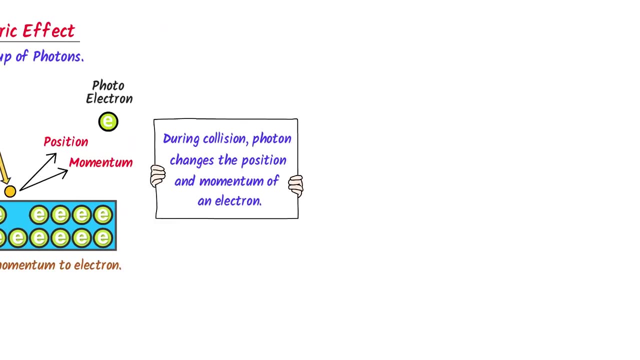 It doesn't change momentum of macroscopic particles like ball. Believe me, if you do not know this concept, you do not understand the Heisenberg Uncertainty Principle. Therefore, note it down, this important concept. Now let me teach you that what is certainty in physics? 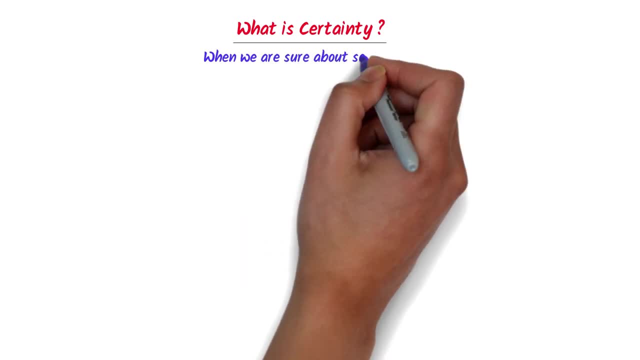 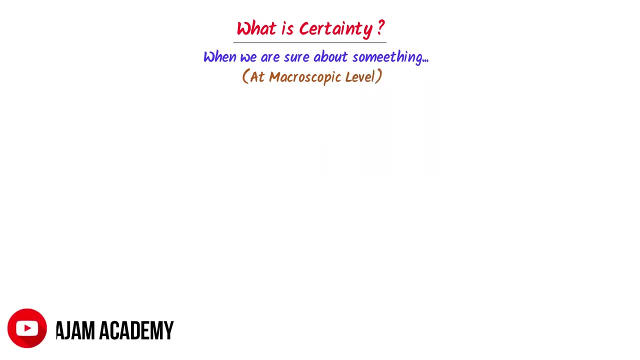 Well, certainty is nothing. but when we are sure about something to happen or occur, we say that it is certain or there is certainty. In physics, at macroscopic level, usually certainty exists. For example, consider a moving car. Let the initial velocity of this car is 10 m per second and its acceleration is equal. 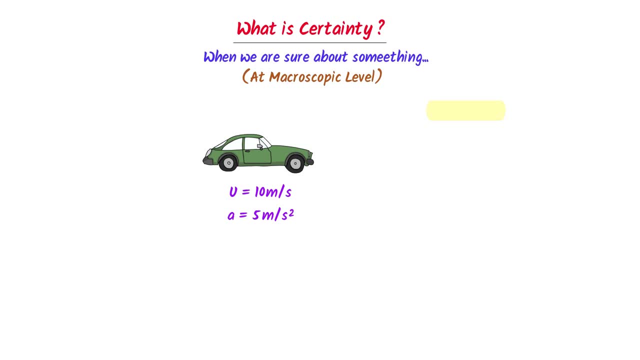 to 5 m per second. Now I am interested that after 2 seconds, what will be its velocity or motion And what will be its position? Well, the answer is simple. Using this equation- vf is equal to vi plus at- we can easily calculate its motion after. 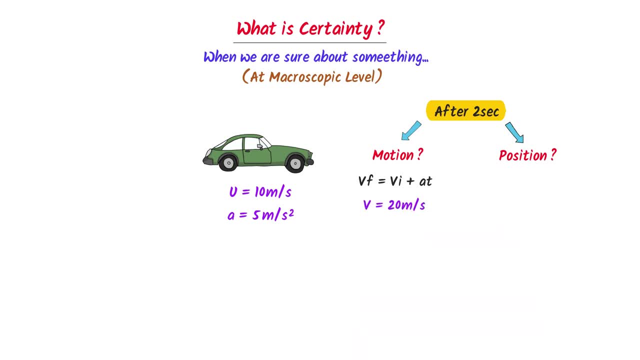 2 seconds, It will be 20 m per second. Secondly, we can easily calculate its position using this equation: 2as is equal to vf square, minus vi squared, It will be 30 m. So we are sure or certain about the motion and position of the car after 2 seconds. 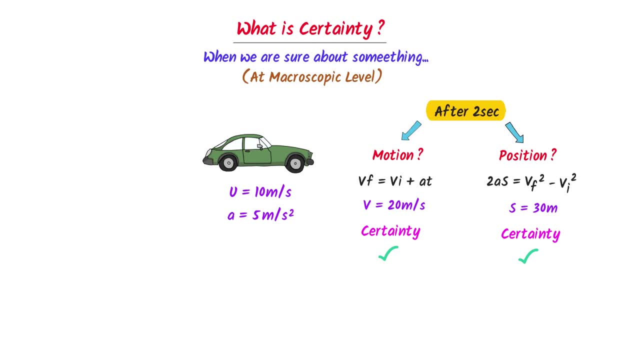 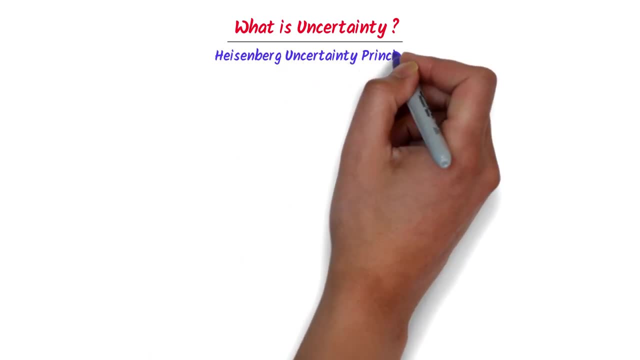 Hence this is the whole concept of certainty in physics. Now, what is uncertainty in physics? The simple and funny answer is Heisenberg Uncertainty Principle. Now I will explain one topic which will cover our three topics, or three questions like uncertainty in physics. 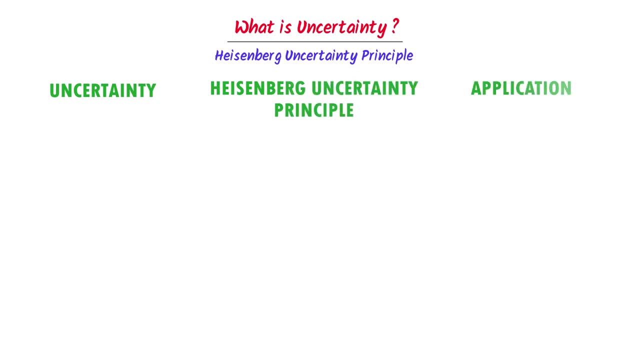 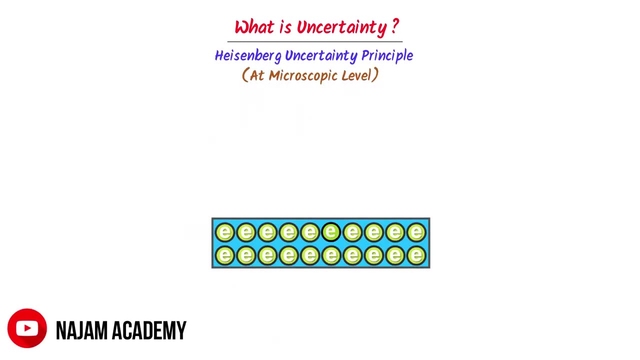 Heisenberg Uncertainty Principle and Application of Heisenberg Uncertainty Principle. Now consider the photoelectric effect, which we have already learned in the previous slide. Let I am interested to find the position and then motion of this electron. But here are two big problems. 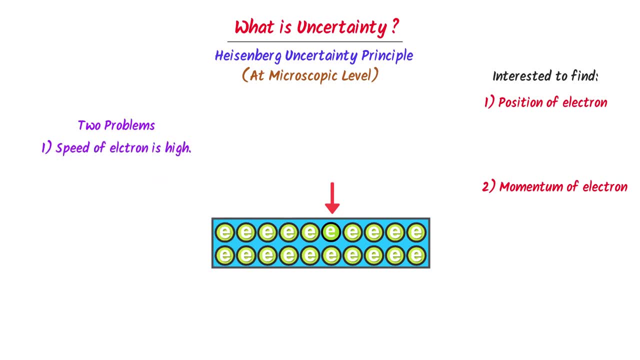 Firstly, speed of electron is approaching to the speed of light. Secondly, Divering Collision Photon of the light changes the position and momentum of the electron. Now I will incident the light on the metal surface. I will quickly note down the position of the electron. 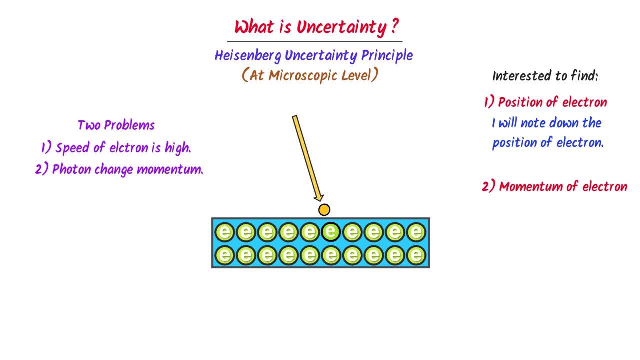 But here is the problem: The photon of light will suddenly collide with the electron. Due to this collision, photon will change the motion or momentum of electron so abruptly that I cannot predict its motion or momentum, Because we know that electron moves with the speed of light. 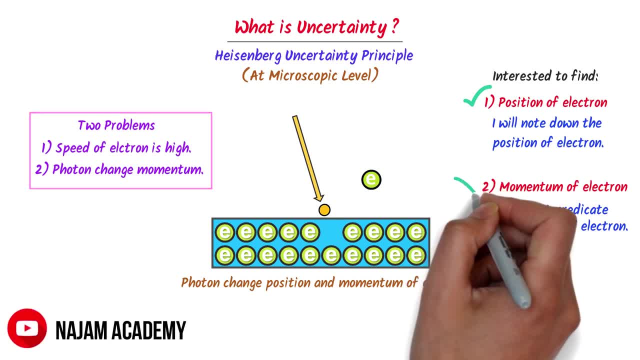 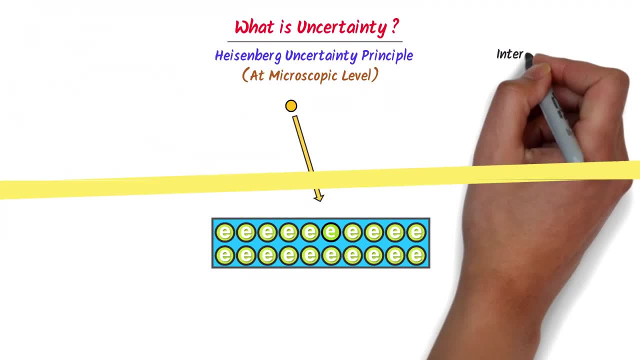 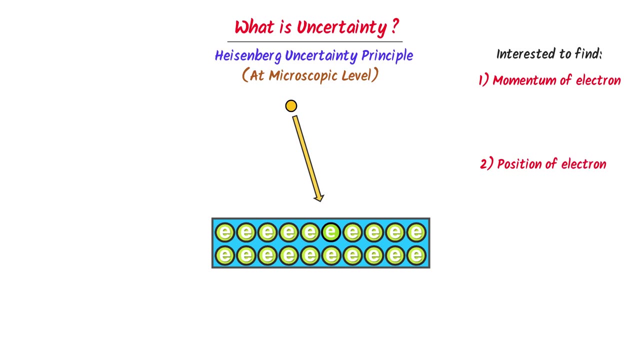 Thus I only measure the position of electron, but I am uncertain, or not sure, about the momentum of electron. Secondly, I am interested to find the motion and then position of electron. Now I will again incident the light on the metal surface. I will quickly note down the motion or momentum of the electron. 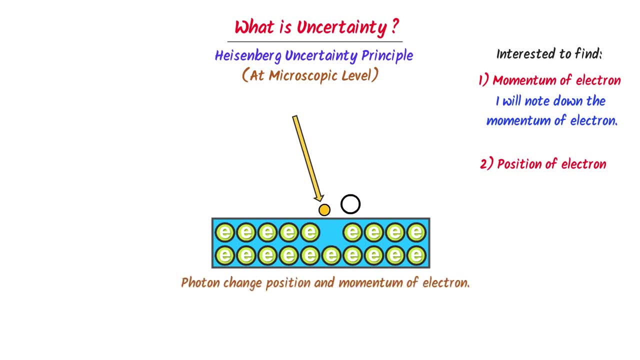 But the photon of light is moving with the speed of light. The photon of the light will suddenly change its position, and I will not be able to predict its position, Because we know that electron moves with the speed of light. Thus, here I only measure the motion or momentum of electron. 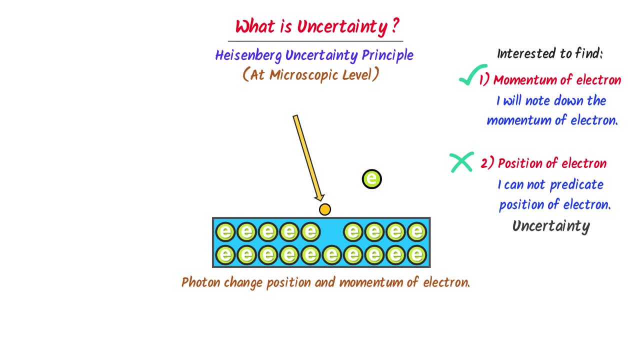 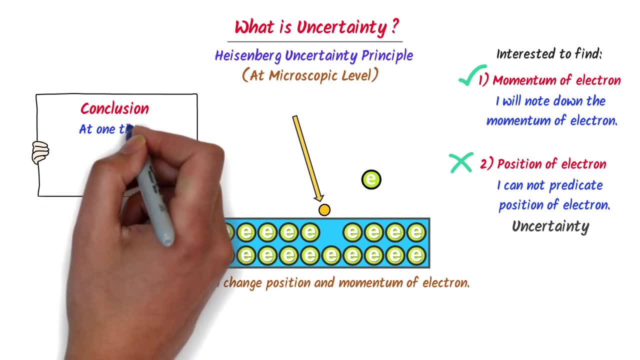 But I am uncertain, or I am not sure about the position of electron. Therefore, overall, we draw this conclusion that at one time we cannot find position of electron. Therefore, overall, we draw this conclusion that at one time we cannot find position of electron. 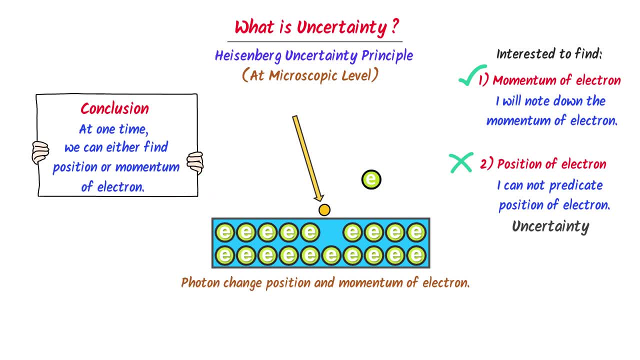 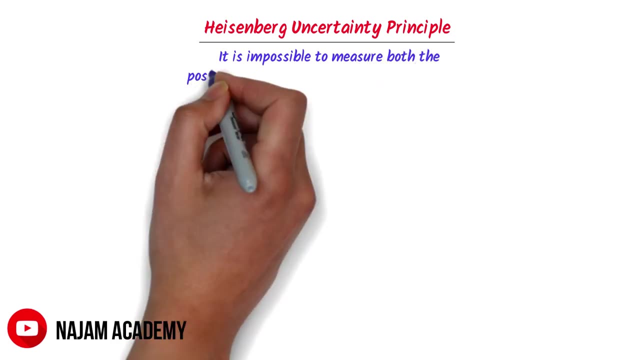 If we have already understood the position and momentum of electrons simultaneously. so this is the whole concept of uncertainty, or this is the concept of Heisenberg uncertainty principle. Therefore, Heisenberg Baba states that it is impossible to measure both the position and momentum of microscopic particles. 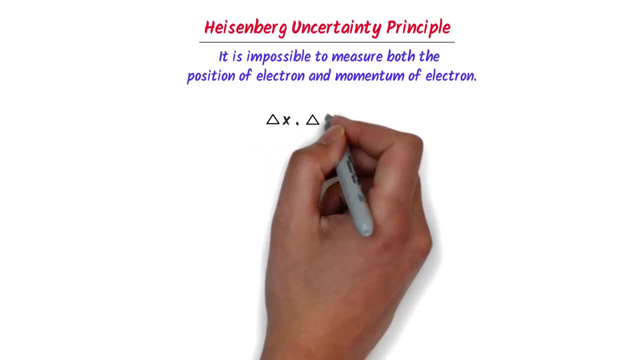 Or we can write del x into del p is greater than or equal to h upon 4 pi. Here we can write del x into del p is greater than or equal to h upon 4 pi. Here we can write del x into del p is greater than or equal to h upon 4 pi. 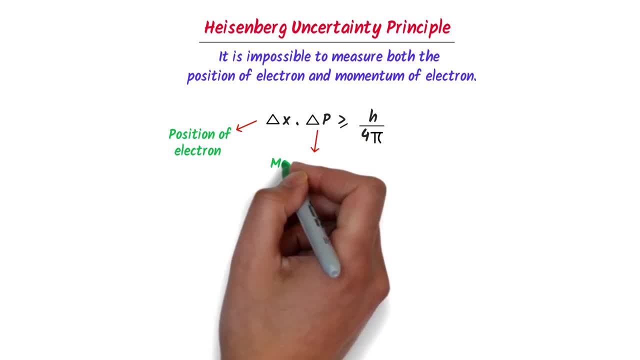 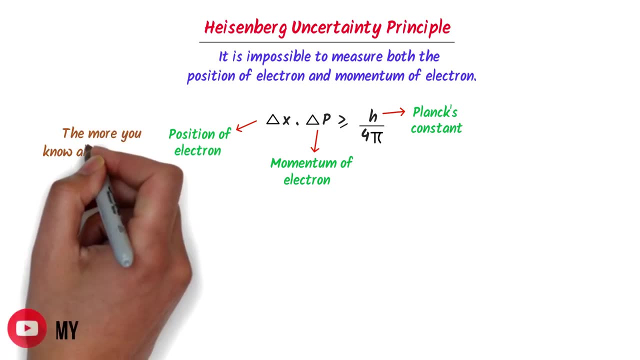 del x is the position of electron, del p is the momentum of electron and h is the Planck's quantum. We can also say that the more you know about the position of electron, the less you know about the momentum of electron. Or we can also say that the more you know about the momentum 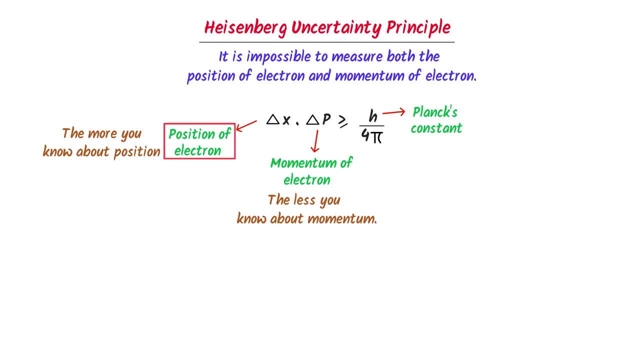 of electron, the less you know about the position of electron. So this is the whole concept of Heisenberg Uncertainty Principle. 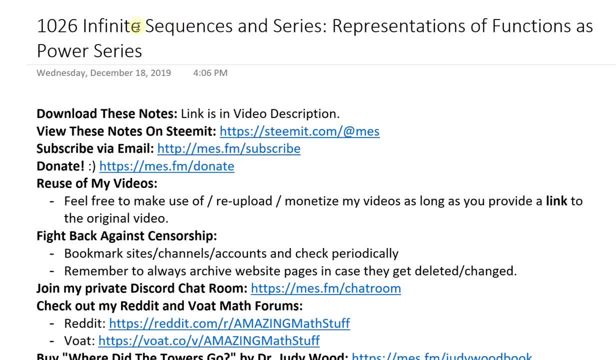 Hi, it's time for another math easy solution. Today I'm going to go over further into infinite sequences and series and this time look at representations of functions as power series, and this is one of the most important concepts in all of calculus and, in fact, all of science. 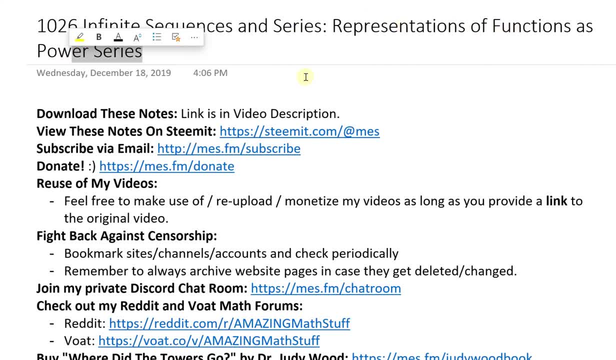 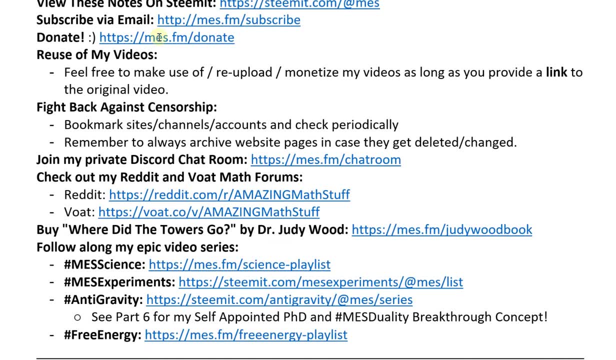 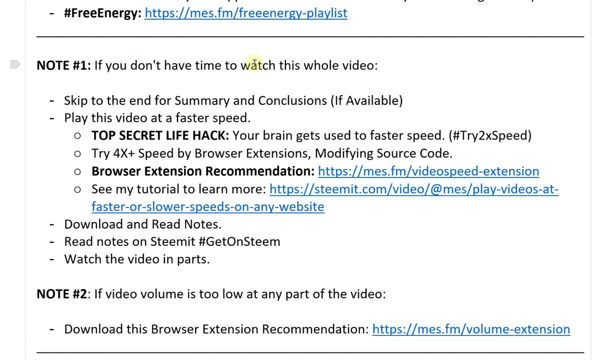 because the ability to represent functions as these power series allows for much easier computation and it's pretty much used throughout physics and science and whatnot. And note, as always, because it's gonna be another epic long video, so if you don't have time to watch this,